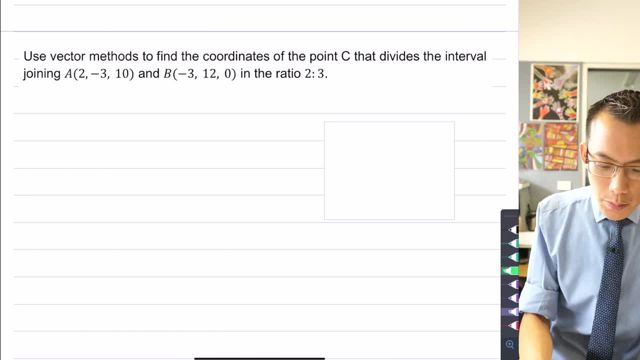 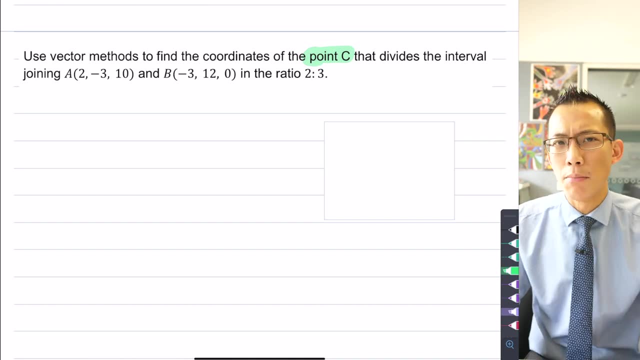 and the clue that tells you that is that really this question is about finding some point C and what you're dividing. this is the clue, like if you're wondering, how do I know when it's important to have my coordinate system set up and have all my three axes and when is it not important? Well, 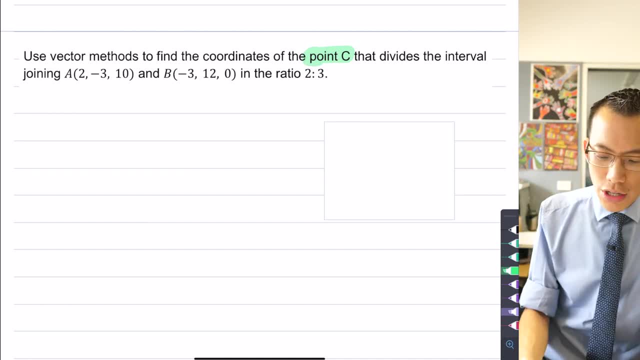 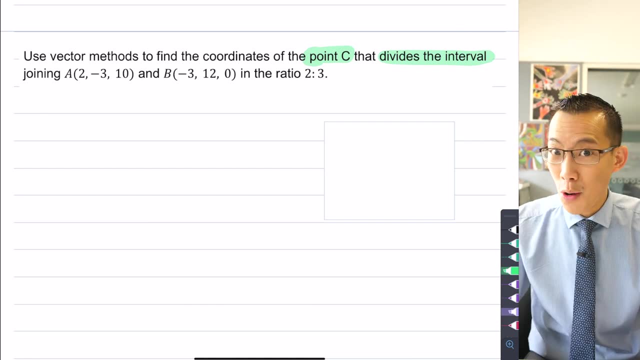 have a look at what the question requires of you. You're finding point C, which is dividing an interval right Now. an interval is in fact itself a one-dimensional object that you can understand in two dimensions. Just if I pick out two points, A and B, and then just join them. 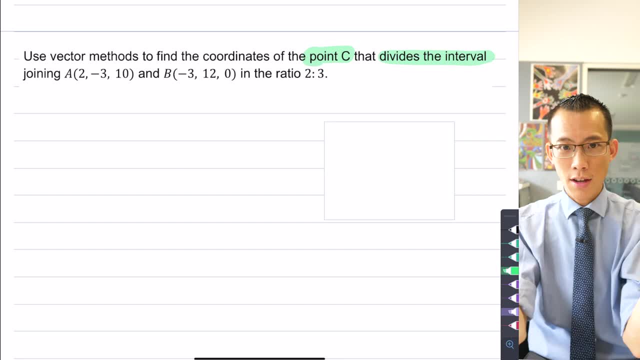 together with an interval, then you can see that it's a one-dimensional object. So if I pick out point C, I can just think of that only in a two-dimensional sense. So therefore a three-dimensional diagram isn't necessarily going to help you here. How do I then represent what's going on between A? 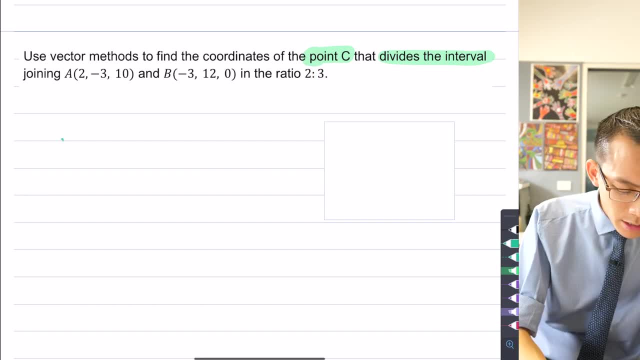 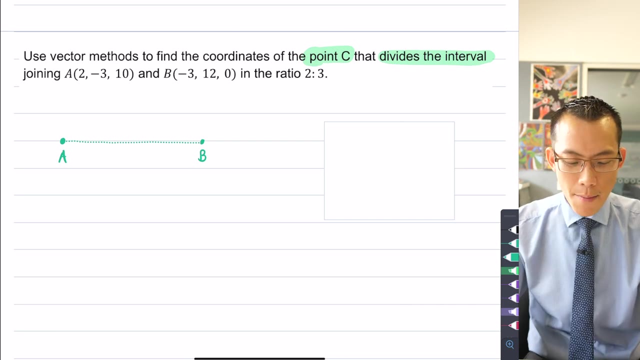 and B and this ratio division. Well, if we set out some arbitrary A and another arbitrary B, we have an interval joining these two and I can sort of represent it like so. And to divide this interval into the ratio two to three means that I'm going to pick out markers. 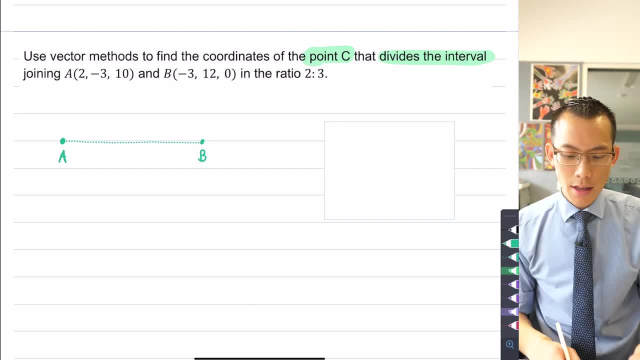 such that when I put point C on one of those markers, then the ratio between the left-hand side and the right-hand side will be two to three. Now, if you want one component to be two and the other component to be three- that's the ratio two to three- then you're obviously going to need five. 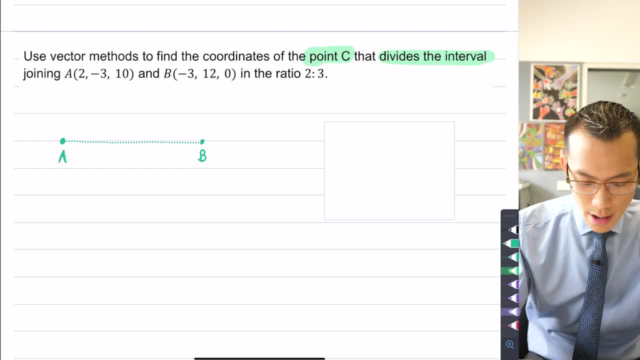 components- in total five parts. So let me show you what that looks like. If I were to try and divide this up into five equal sections, I think it would look something like that, And what I could say is: well, if I highlighted this section here. 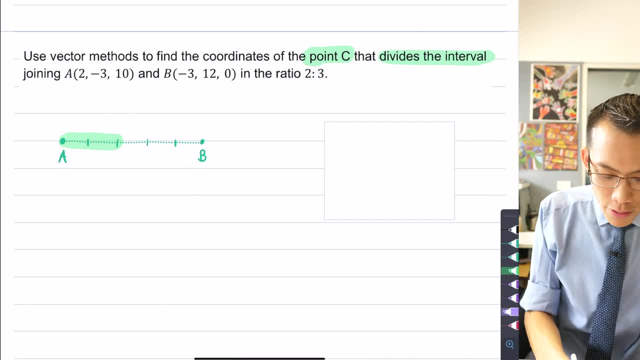 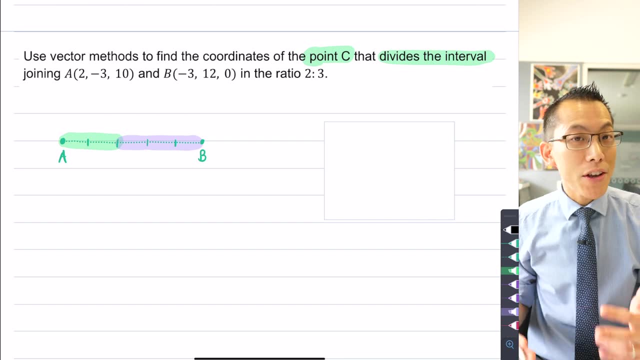 it would be in a ratio of two to three, with this other section over here, So you can literally see the two to three ratio there. okay, Now what we're trying to do, therefore, is to find that point right in there, right in there, and that'll be our point C that divides the interval accordingly. So, 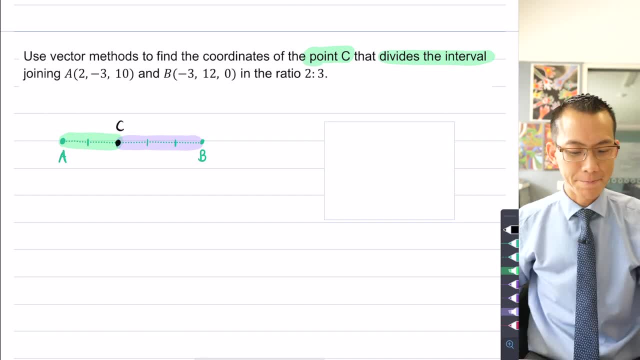 I'm going to put C right there, okay. Now, how do we use vector methods, as the question has specified, in order to find points? Well, if you have a think about this and you think about the arithmetic of vectors that you know about, 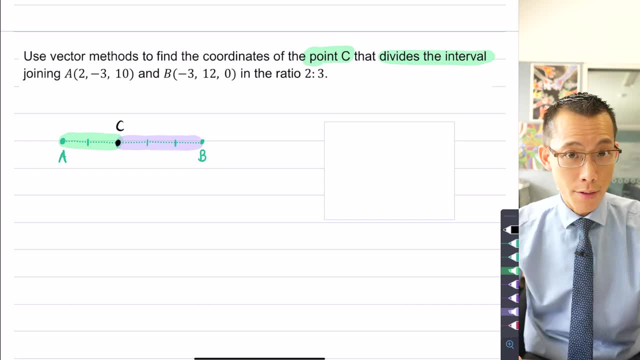 the thing that can help us here is the scalar multiple of a vector. If we, for example, could say: we know what vector AB is. Let me put it across the top in green: right: Vector AB. right, The way you could find. 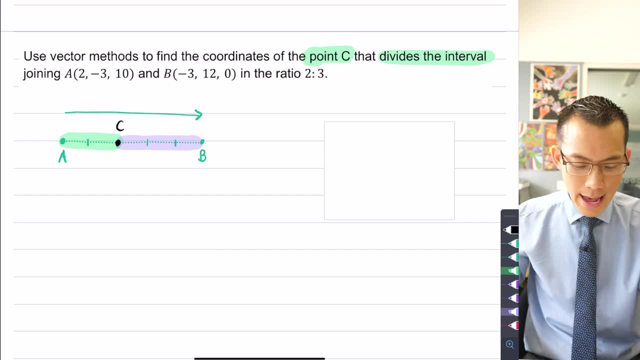 C is to say, well, if you start from A and go some proportion of vector AB- I should say vector AB, I should have labeled that This is what we would call AB. If you can find the correct proportion of vector AB, then that'll take you straight from A to C. Or, of course, you could go from B to C if you. 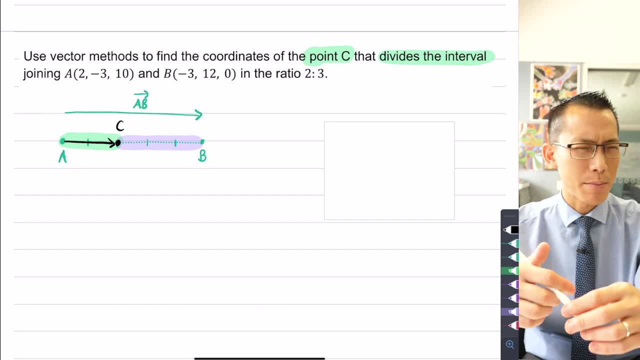 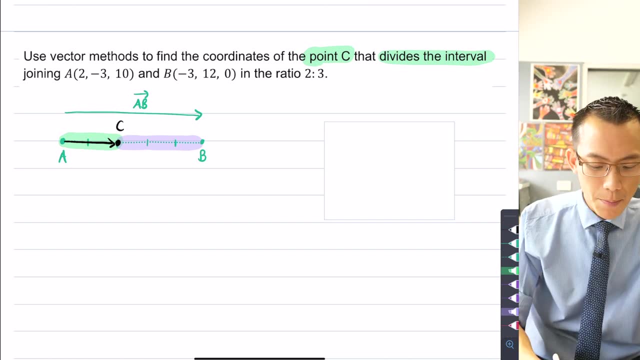 like, but AC is in the same direction as AB, so it seems more sensible to start from A. Now, how would you do that? Well, again, I mentioned it's with this scalar multiple of a vector, Because I've divided up this whole interval into five equal parts, and what I want is this part here which is: 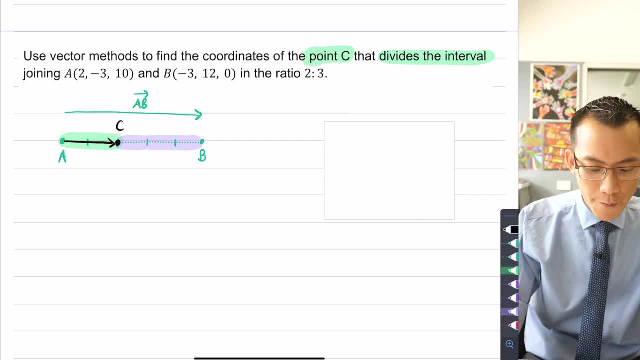 two-fifths of the A vector. I want to create a vector from this whole interval, And what I want is this part here of the entire interval. Therefore, vector AC is equal to literally two fifths of vector AB. 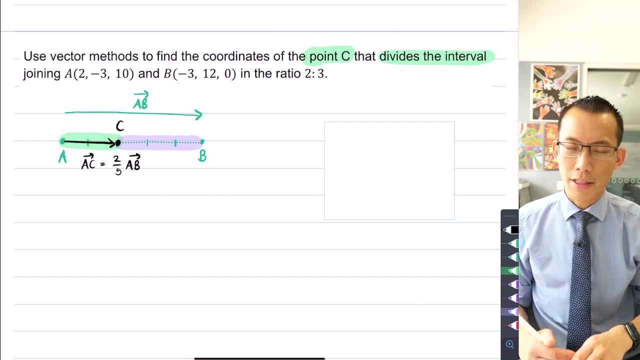 You see that It's going in the same direction. The scalar multiple out the front there, that coefficient doesn't change the direction. it just changed the magnitude right, Which is exactly what we want. We only want two fifths of the magnitude. 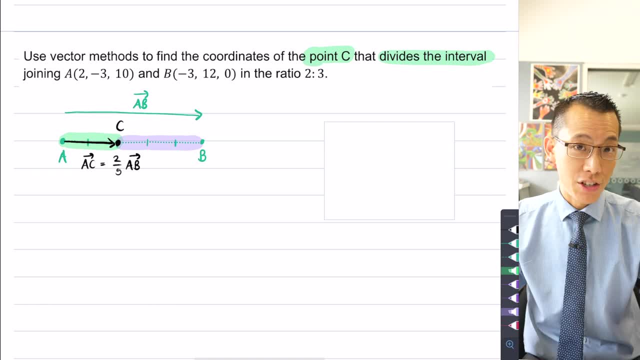 that will get us this two to three ratio. So in order to find AC, which will give us the coordinates of C, what I need first is to find AB, and then I can use that as my stepping stone. So that's going to be our path to this question. 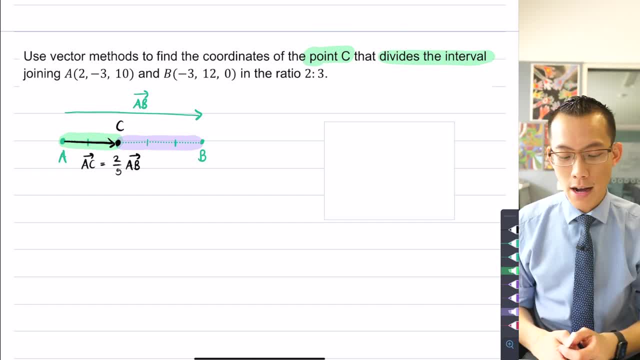 I'm going to find out what AB is, because that vector is not provided in the question. I need to work out what it is. Then I'm going to use AB to work out AC, And once I do that there's just a little bit of legwork. 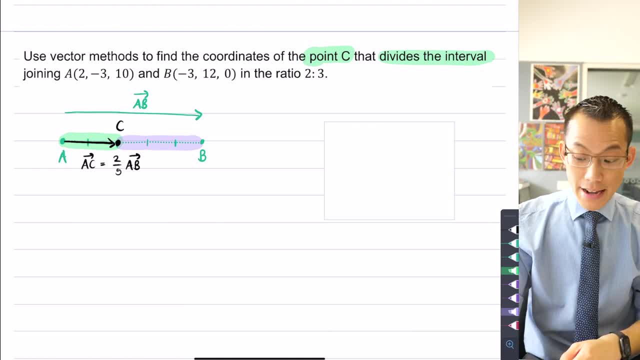 to work out the coordinates of C. So that's where we're going to go Now: to work out what the vector AB is equal to. in terms of the vectors I already know because I've got a, I can say I have a position. vector for A. 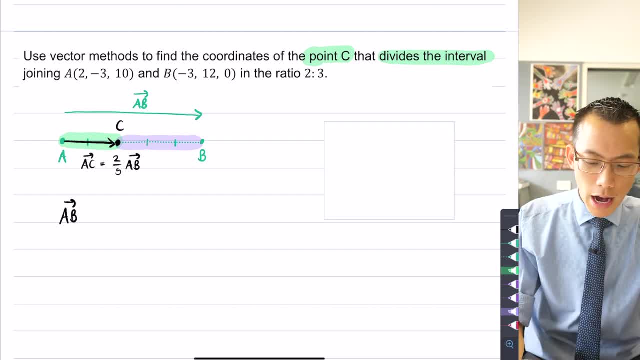 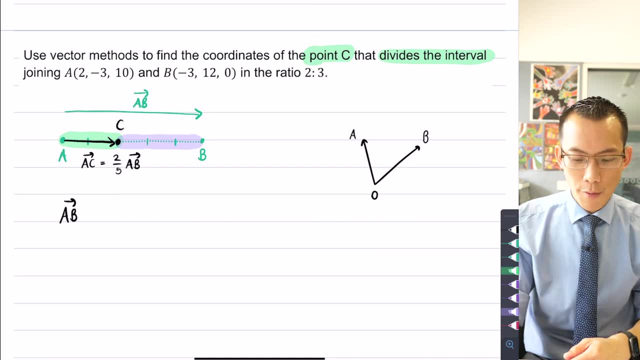 and I've got a position vector for B based on their coordinates. Again, a handy diagram will help you out here, right? So what I do is I consider the position vectors for each of these, A and B, relative to the origin. 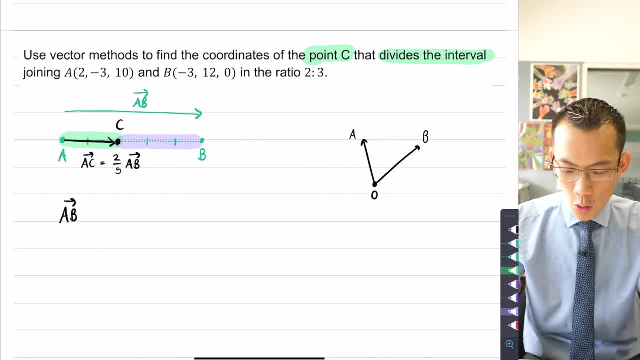 So if I'm starting here at the origin, I can say: well, OA is going to be going in that correct direction. by the way, is going to be the vector two negative three, 10, column form. In fact, I could even write it like so: 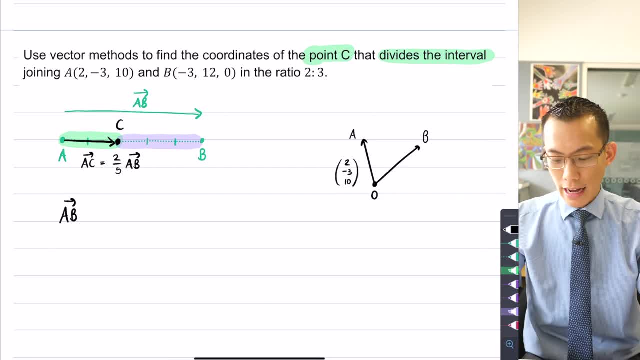 two negative three and then 10.. And I guess I could call that, you know, little A, with the little tilde underneath it, And then little B, vector OB is going to be. let's have a look here. I've got negative three and then 12,. 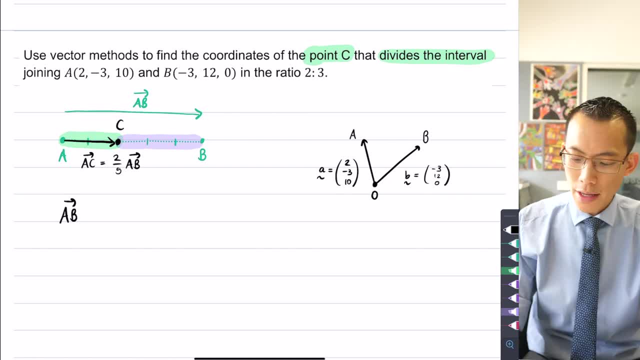 and then zero is my Z vector there. Now, in order to get AB, which you can see, I guess we would represent, I used green before, didn't I Like? so This is the AB vector. This is the Z vector. 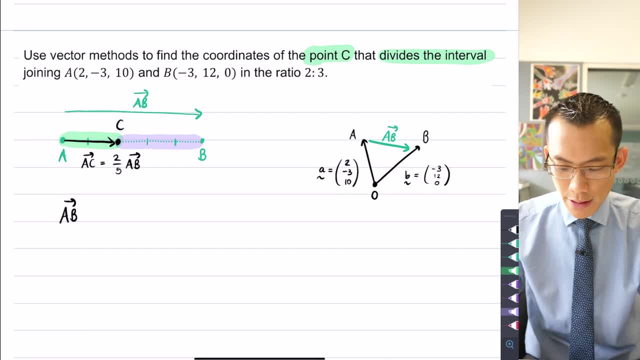 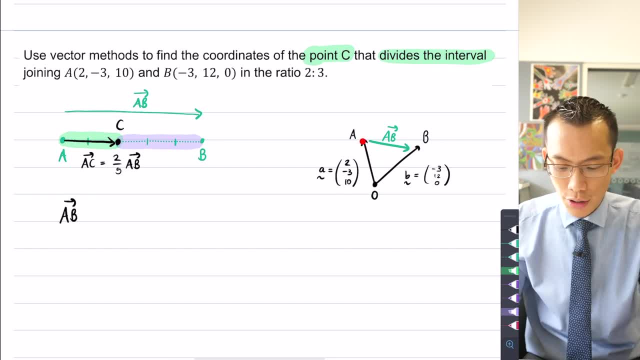 The way that I can compose the vectors I already know is to go backwards, not from O to A- this will take me from O to A- but to go from A to O and then O to B. So this is the set of vectors. 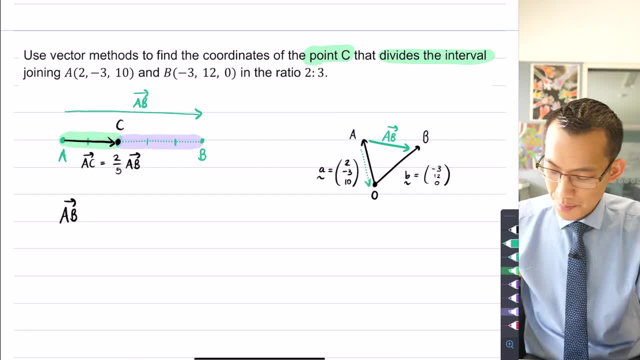 that I'm going to string together right A to O and then O to B, And you can see here, if I'm carrying on this color here to go from A to to O will be negative of this little A vector. 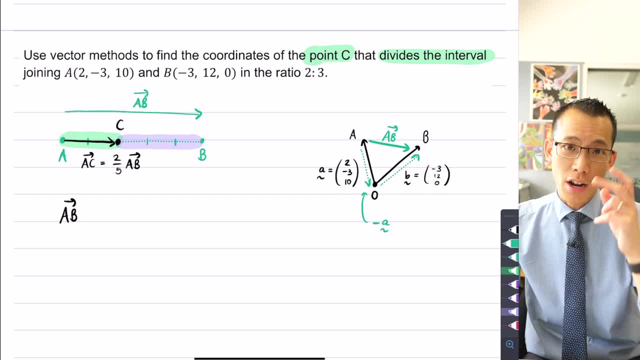 because I'm going in the opposite direction. Magnitude: same direction. I'm just going to flip all of the signs. So, therefore, what I can say is: AB is going to be equal to what did we say? AO plus OB. 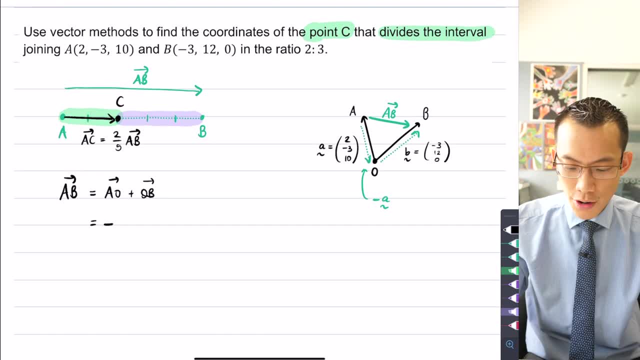 But what that's really equal to is negative of what I know little A vector is going to be. So really that is, let's see here, negative. oh sorry, I've already put the negative out the front. two negative three: 10,. 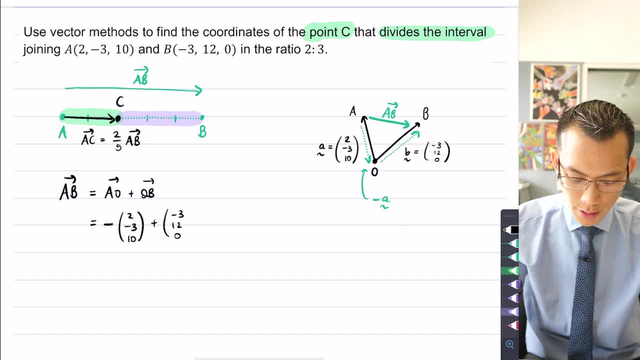 and then I'm going to add negative three, 12, zero. So if you wanted, some people are going to go straight to that vector and say it's going to be OB. take away OA. I haven't written it like that immediately because it sort of seems weird to say OB. 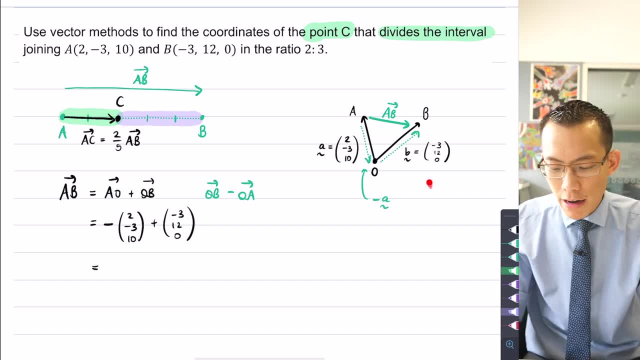 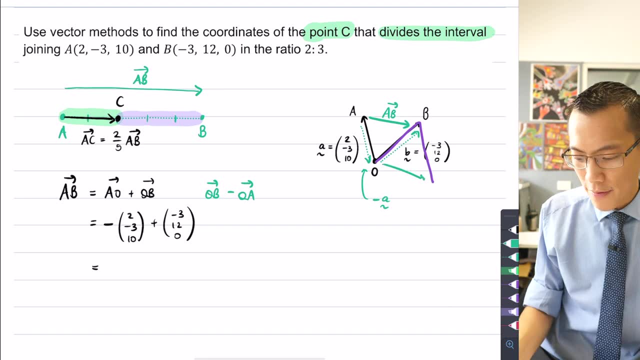 and then do OA, which actually sends me over here because of the parallelogram law. if you think about what happens when you go here, here and then here, you are going to get the same AB vector over there, just translated elsewhere. 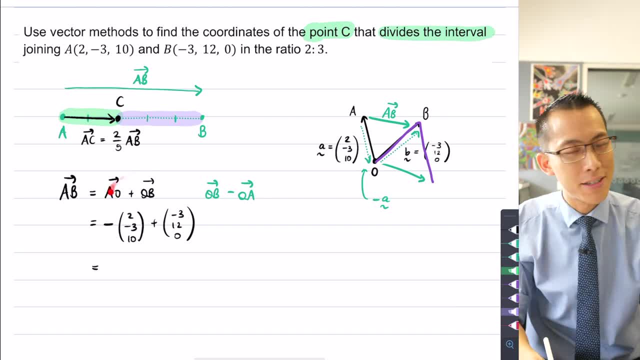 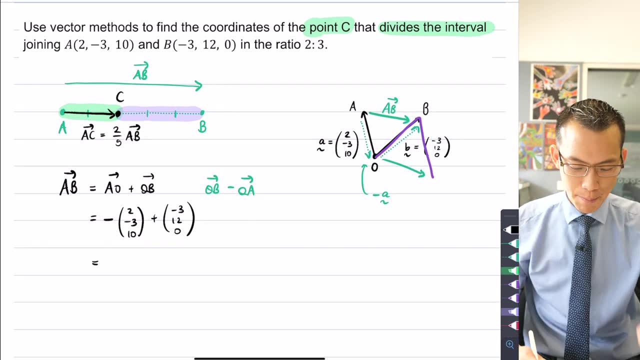 It's the opposite side of the parallelogram, But I think this is a more helpful way to see what's going on using vector methods, right, Okay, so now that I've got my vectors down, we can actually go ahead and we can compute this. 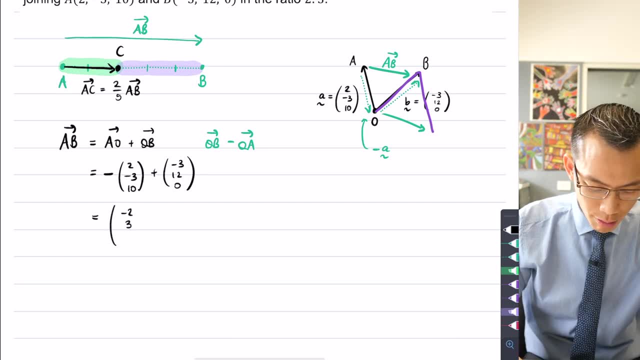 So what do we got? I'm going to have negative two, three and negative 10.. And then what I'm adding is this: negative three, I'm going to add 12, and then it comes to zero along the end here. 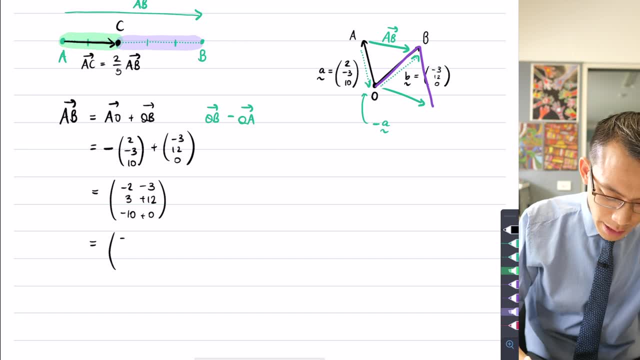 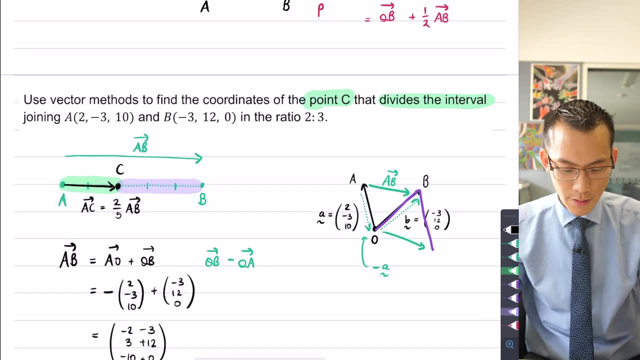 Okay, what does that give us? Well, it looks like I'm going to get negative five. I've got 15 in the middle there and then negative 10.. Okay, let's have a quick look. That all seems fine to me. happy times. 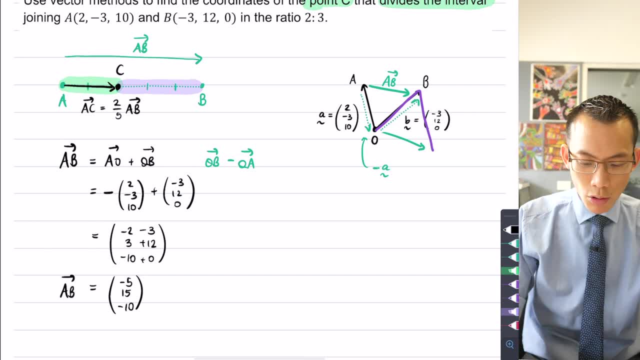 So what I've got now is vector AB, but you'll recall I didn't want actually vector AB. That was just a stepping stone to get to AC. AC is two fifths of the way from A to B, So all I need to do to turn this into AC. 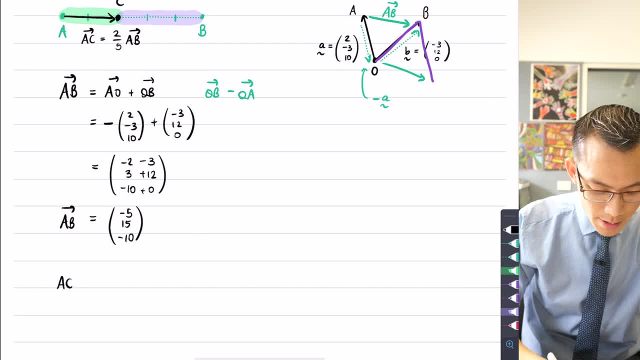 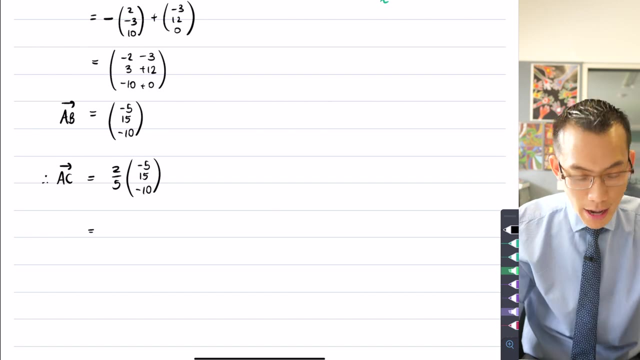 is to multiply it by two fifths. So I can say AC. therefore, this equals two fifths of the vector that we calculated up here. So if we have a think about this, I'm going to be dividing by five, then doubling. 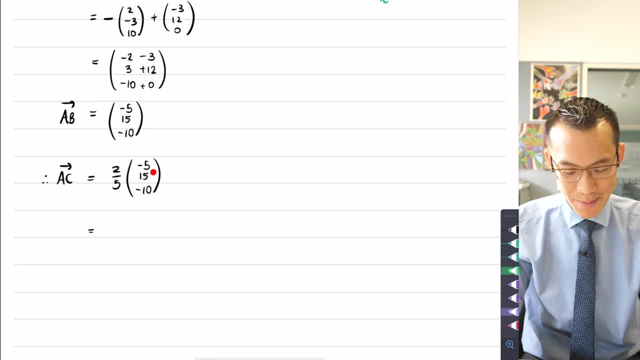 That's not too hard because conveniently, it's almost like this question was designed for this purpose. Everything here is a multiple of five, So if I go ahead and do my scalar multiple, I guess I'm gonna get negative one, two, three, five, squash. 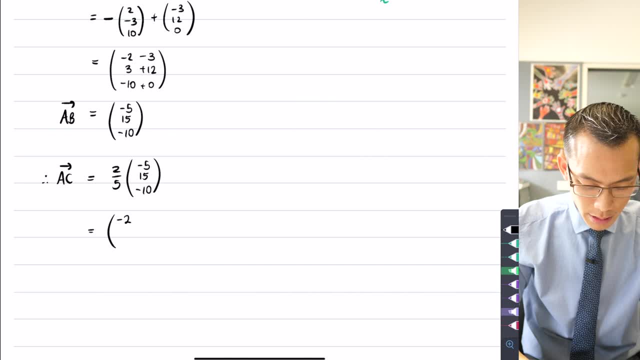 negative 2,, this is going to give me 6, and then this is going to give me negative 4.. Okay, so this is AC, and if you have a think about it, it is: yes, you're going in the same. 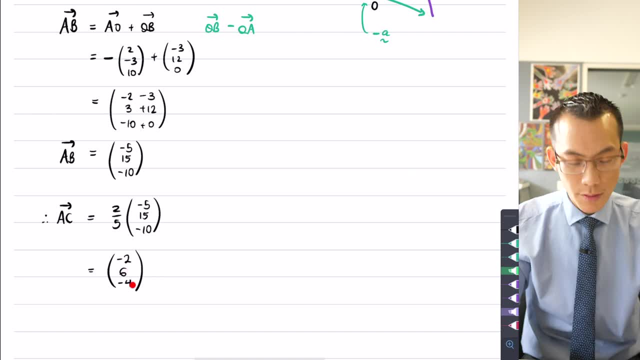 directions: negative, positive, negative, negative, positive, negative. but you're not going as far. you're going two-fifths of the way. Okay, that all looks good to me, but it's still not the question that I was trying to answer. I was trying to find out. well, where is C? This is just how to 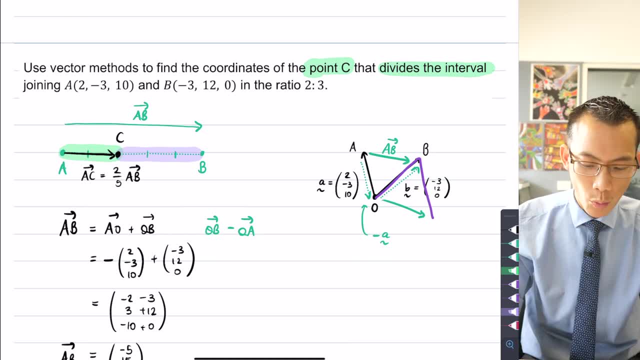 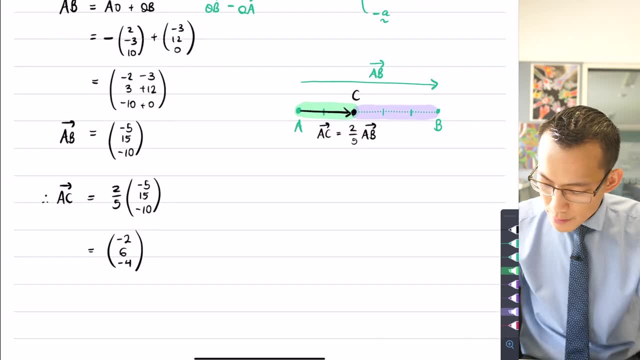 get from A to C. so how do I go further? And the way to sort of calculate that if I bring this over here I can do an extra sort of bit of construction here. I can say, well, let's remember that the origin is somewhere else in space. To get to C, to work out what that vector will be, 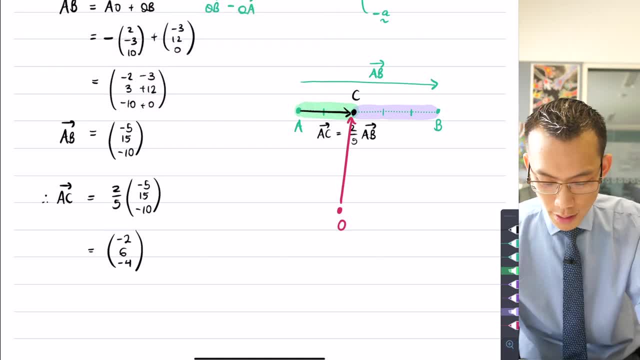 I can do that in two pieces, right? I can go first, first, and then I can go second, and then I can go third, and then I can go third, and then I can go third, and then I can go fourth, and then I can go fifth, and then I can go sixth, and then I can go. 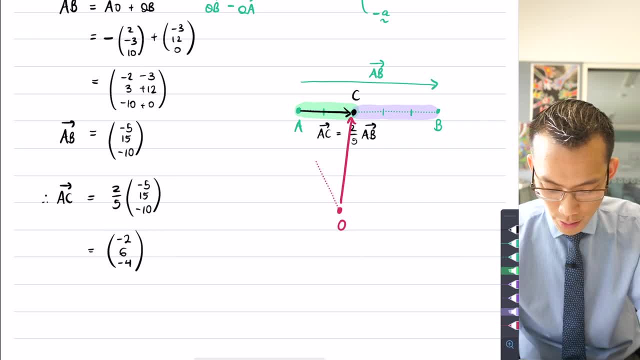 I should start from O, shouldn't I? I can go from O all the way up to A and then A over to C, which I've already calculated. So really, what I want to get to the coordinates of C is to do O, A. 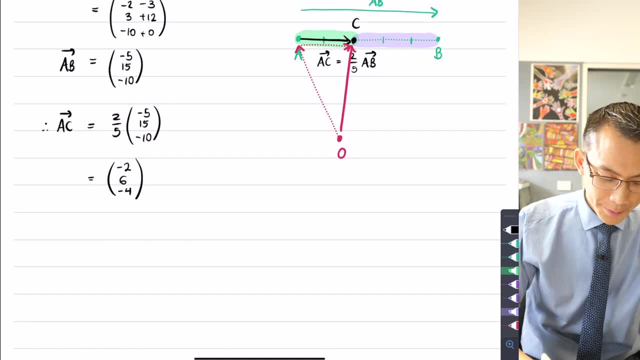 and then add A C and that will get me there, So I can say O C. maybe I'll say I have a logical conjunction there. but O C equals go to A first and then go from A to C, and I know what all of. 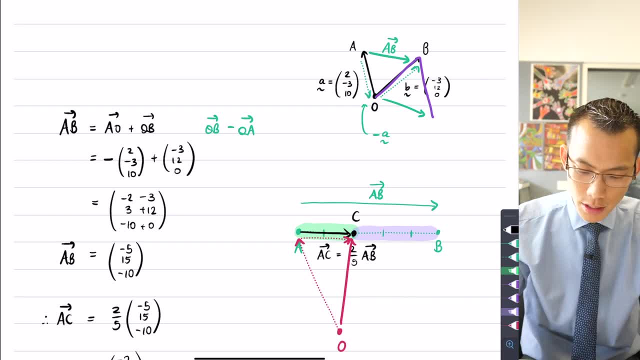 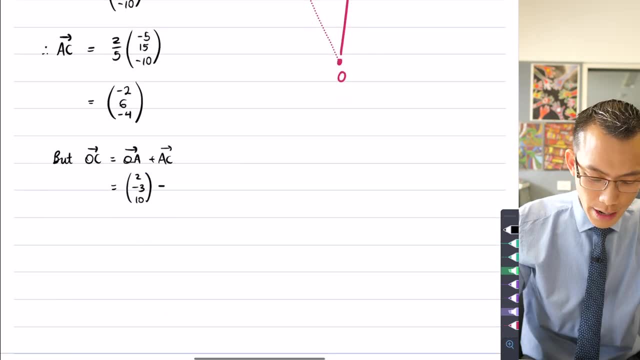 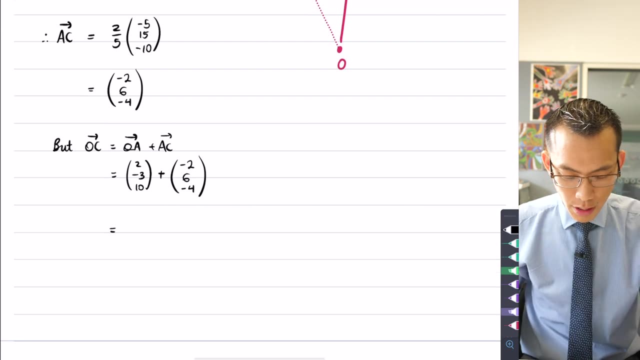 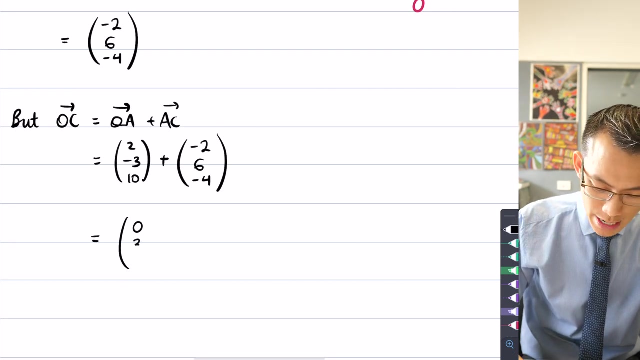 those individual components are O. A. of course is this original vector here. Let's just grab that, And then I'm going to add on what I just found over here. So what's that going to be equal to? It looks to me like I'm getting zero, three and then six. Zero, three, six. Those are my coordinates. 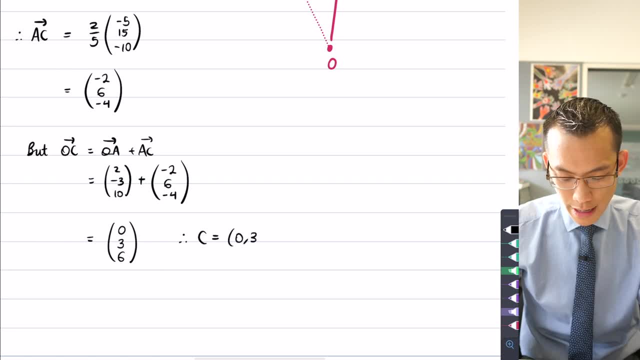 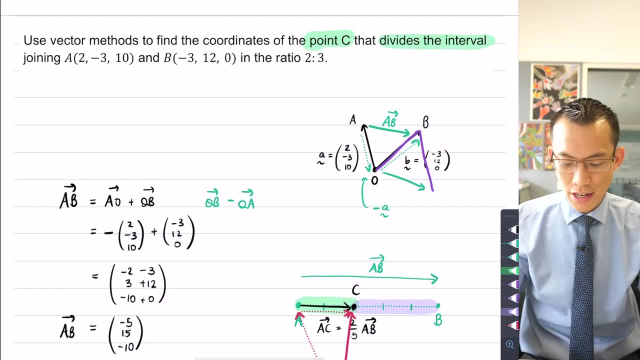 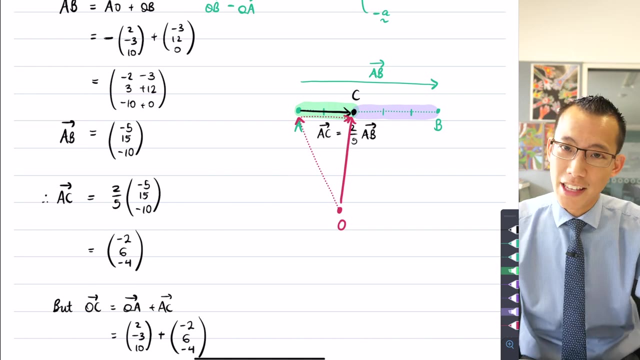 I can say: C equals zero, three six, using vector methods. So I divided up the interval in this particular ratio here, knowing that it'd be two-fifths of the way, and then I just put together my vectors. I composed them in the correct order to give me the coordinates that I was after. 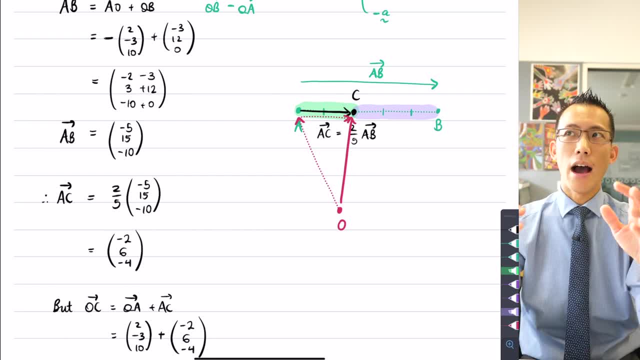 Now, just before we leave off this question, it is worth pointing out that, as with what we've seen throughout the entire topic of vectors- because vectors are defined as direction and they're not going to be the same- they're not going to be the same. they're not going to be the same.